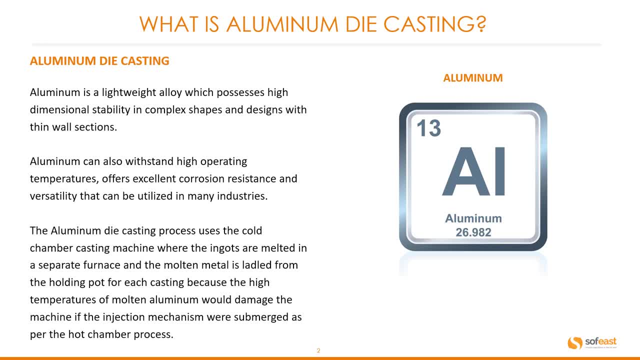 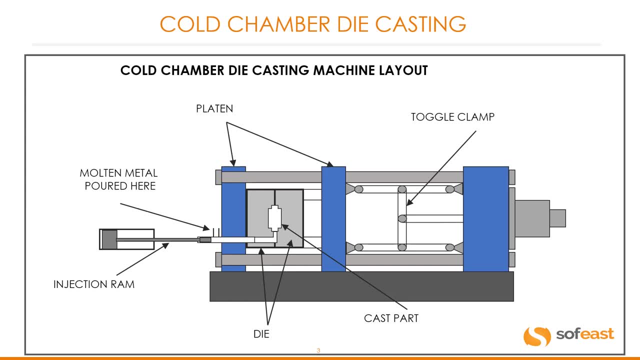 if the injection mechanism were submerged as per the hot chamber process. Here is a cold chamber die casting machine layout. You can clearly see here the platens, the toggle system which closes the die, the die itself, the cast part or in this case, the cavity. 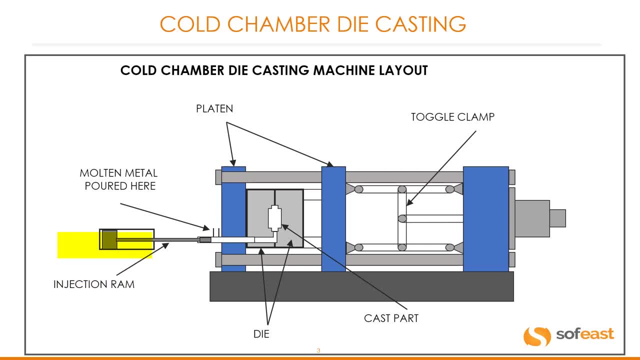 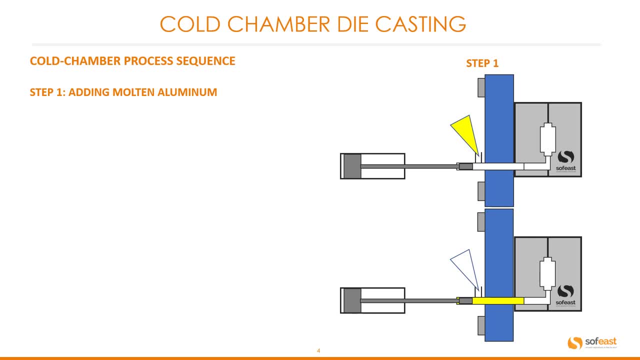 the injection ram system and where the molten metal is poured into. Let's have a look at the aluminum die casting process step-by-step. Step 1. Adding the molten aluminum Before the die halves are shut. die lubrication or release agent is applied to the surfaces. This helps with 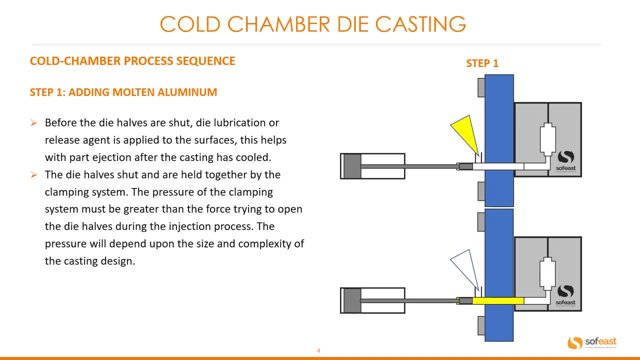 part ejection. after the casting has cooled, The die halves shut shut and are held together by the clamping system. The pressure of the clamping system must be greater than the force trying to open the die halves during the injection process. The pressure will depend upon the size and the complexity of the casting design. 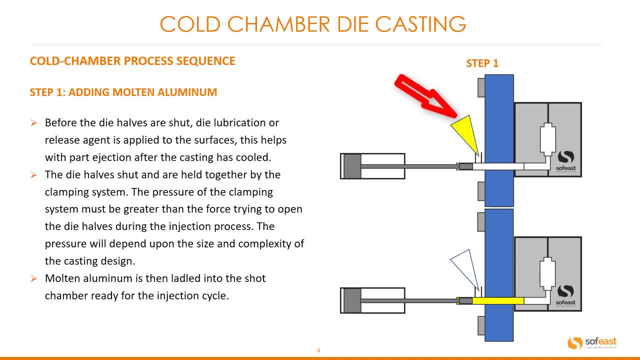 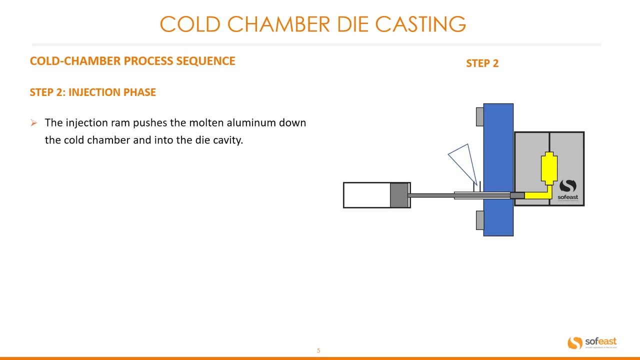 Molten aluminum is then ladled into the shock chamber, ready for the injection cycle. You can see this shown in the image at the top. The molten aluminum fills the shock chamber. This is shown in the image at the bottom. here Step two, the injection phase. The injection ram pushes the molten aluminum. 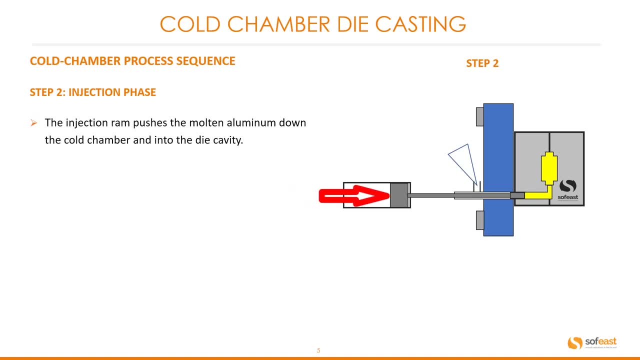 down the cold chamber into the die cavity. The image on right here shows this process. During the movement, the ram seals off the input port. Pressures during the injection phase can be between 300 psi or 1.3 tons up to 50,000 psi. 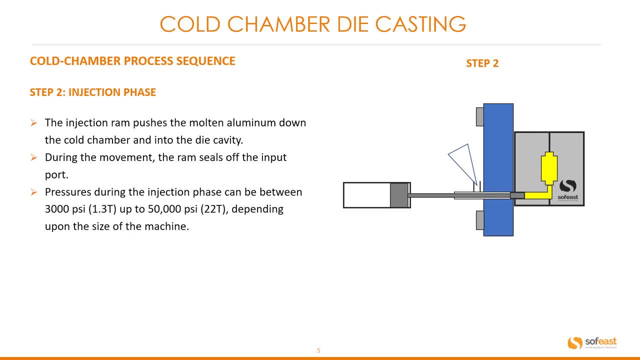 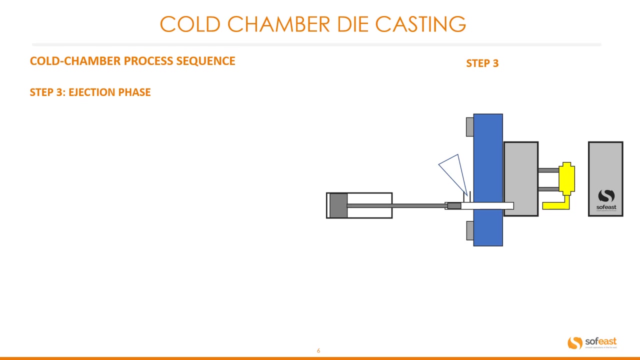 which is around 22 tons, depending upon the size of the machine. Pressure is maintained while the casting is solidifying. Pressure can be increased during this phase to ensure the cavity is completely filled and casting integrity is achieved. Step three: the ejection phase. 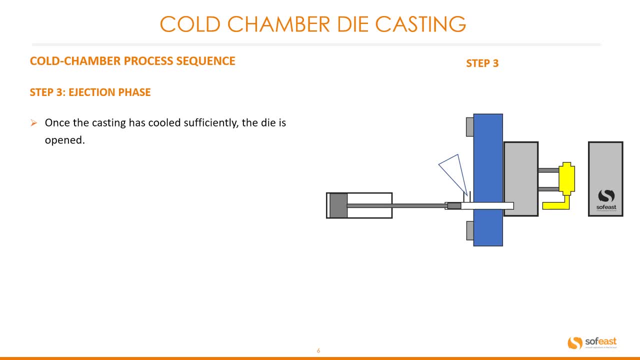 Once the casting has cooled sufficiently, the die is opened. The ejector system then pushes the casting out of the die half. You can see this shown in the image on the right here. During this time, the injection ram is retracted, exposing the input port. 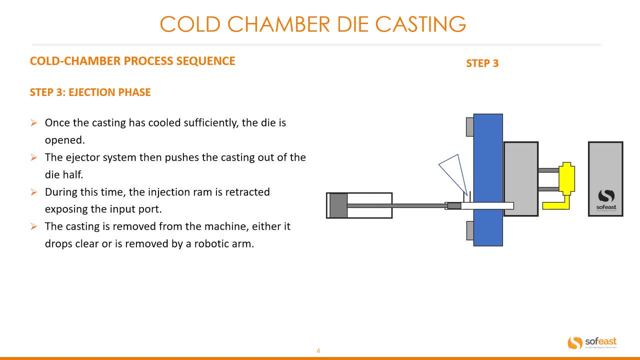 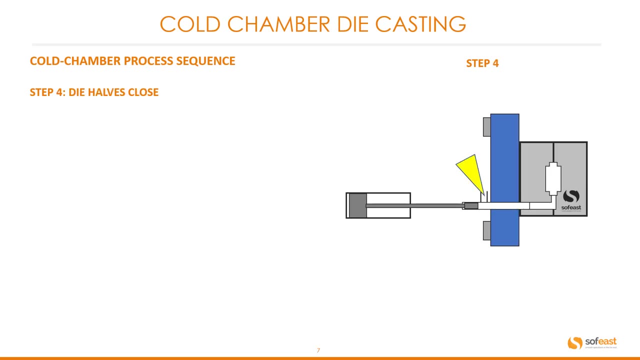 The casting is removed from the machine. Either it drops clear or is removed by a robotic arm. Die lubrication or release agent is then applied to the die halves. Step four: the die halves close. The die half close, ready for the next cycle. 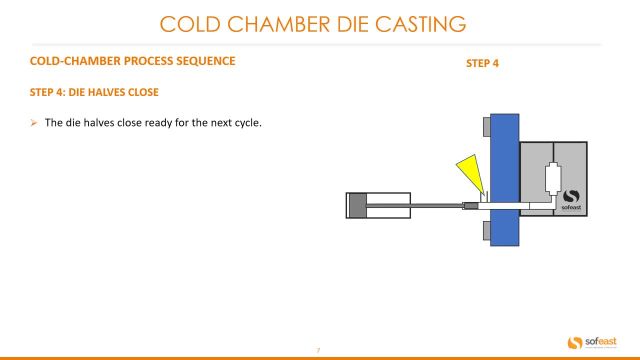 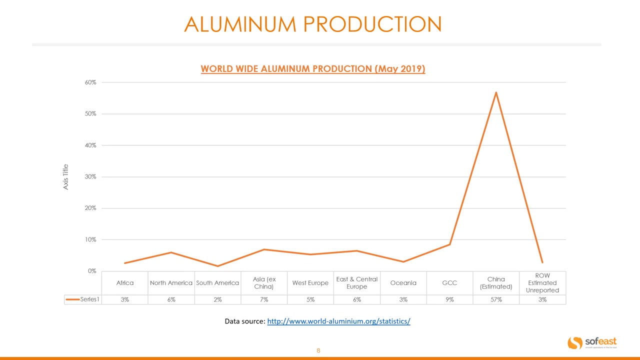 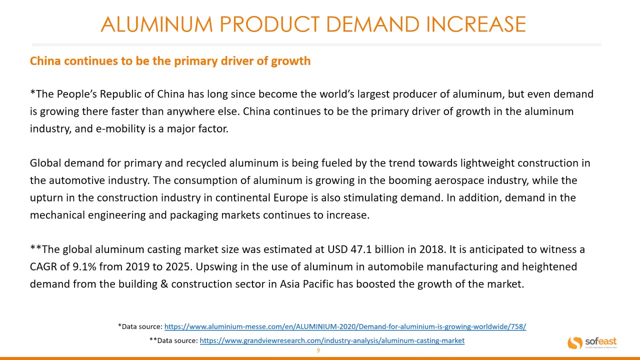 Basically, they are the four steps that complete this cold chamber process sequence. Here are examples of some finished die casting in aluminum. Here are a few facts regarding aluminum production. So this is the worldwide aluminum production data based on May 2019.. You can clearly see that China is dominant in the production of aluminum around the world. 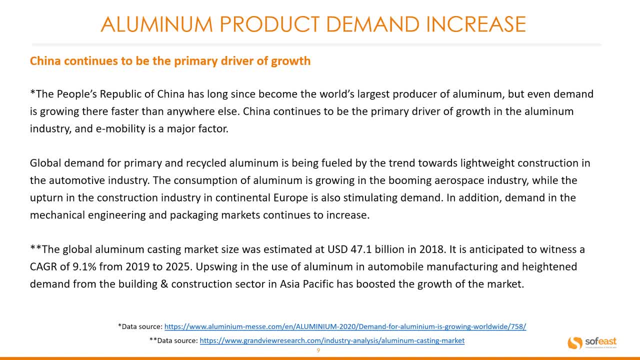 Aluminum product demand increase. So China continues to be the primary driver for growth. So China has long since become the world's largest production of aluminum. But even demand is growing there faster than anywhere else. China continues to be the primary driver of growth in the aluminum industry and e-mobility. 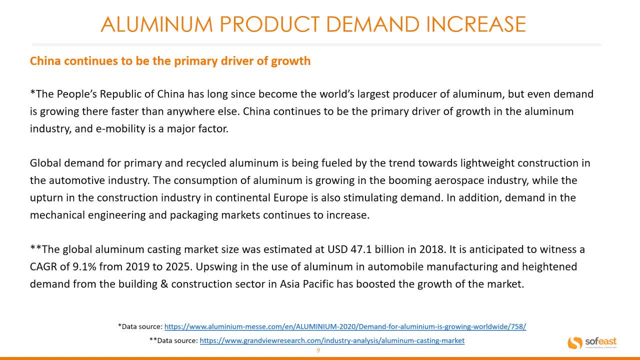 is the major factor. Global demand for primary and recycled aluminum is being fueled by the trend towards lightweight construction in the automotive industry. The consumption of aluminum is growing in the booming aerospace industry, while the upturn in the construction industry in continental Europe is also stimulating demand.